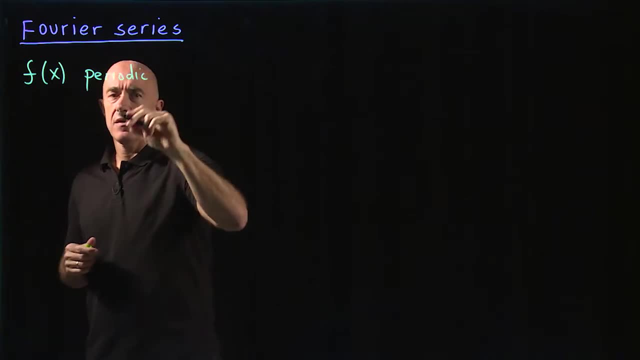 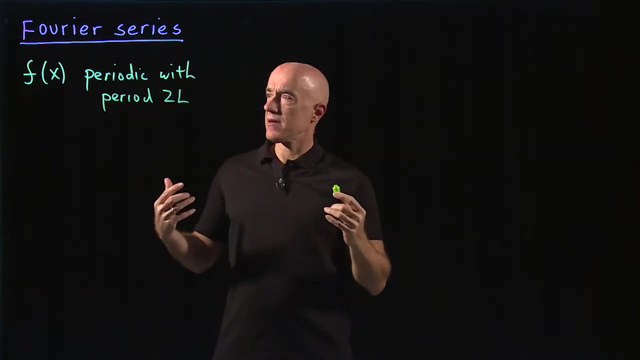 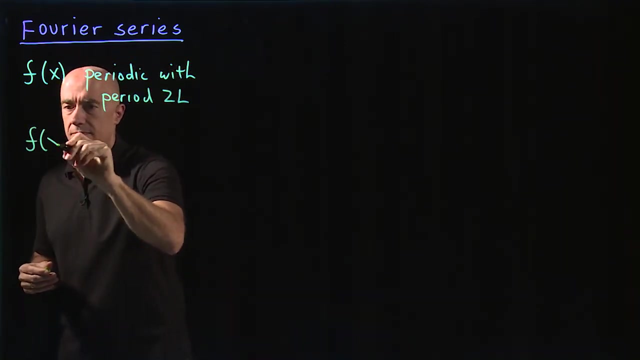 It means it repeats itself every 2L, So periodic with period 2L. How do you represent then f of x as a Fourier series? There's a rather fixed expression for that which I can write down: f of x equals a constant term which we write as a naught divided by 2, plus a series. 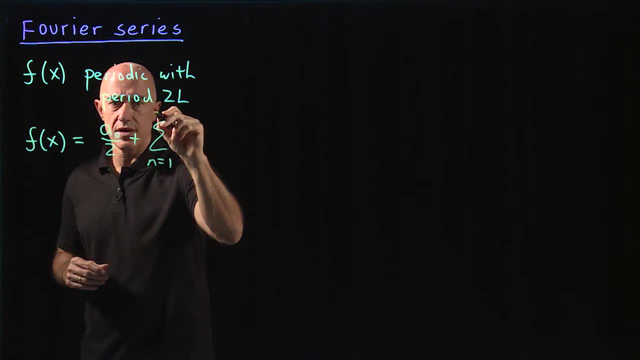 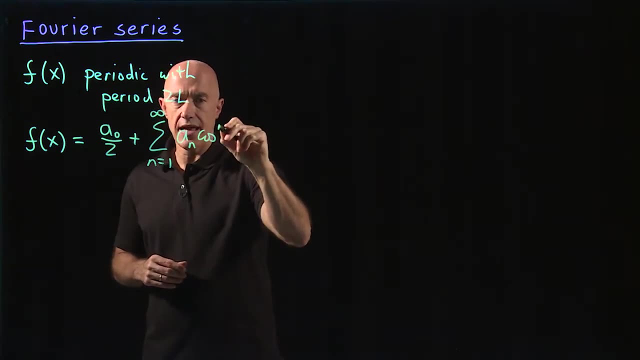 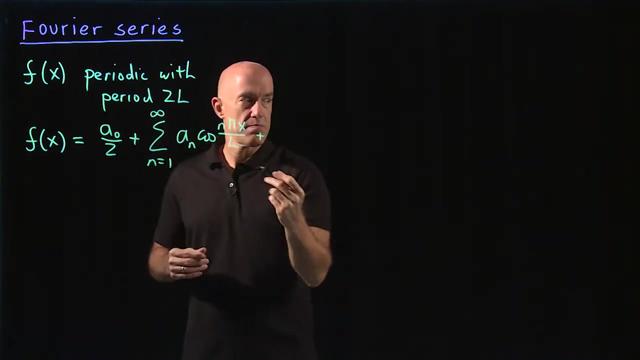 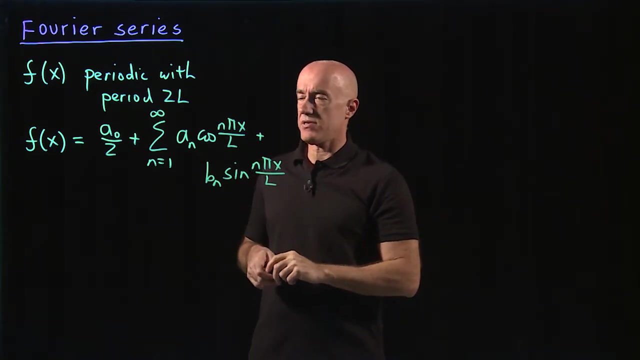 the sum from n equals 1 to infinity of these coefficients: a sub n times cosine n pi x over L, plus b sub n Plus times sine n pi x over L. That's the general form for a Fourier series, The use of the expression cosine n pi x over L, because cosine is a periodic function when x goes. 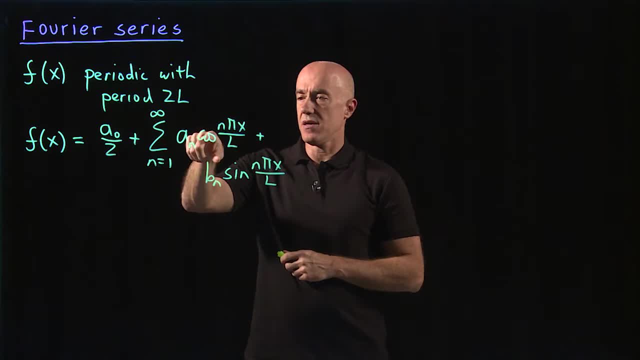 from 0 to 2L, then the cosine function will just repeat itself, And the same for the sine function, So this expression will turn out to be periodic, with a period of 2L. These coefficients, a, naught, a, n and b? n- for n equals 1 to infinity- have to be determined. 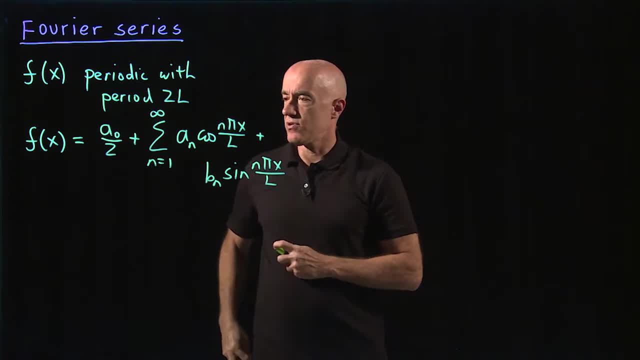 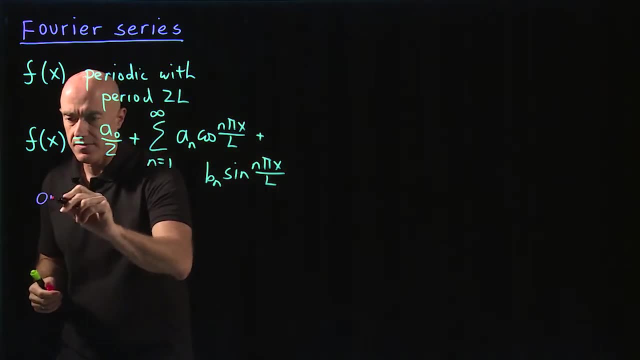 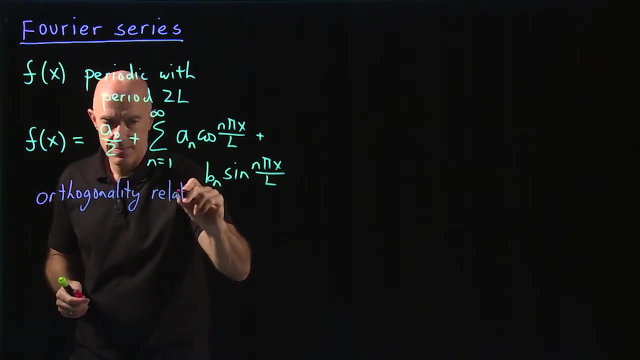 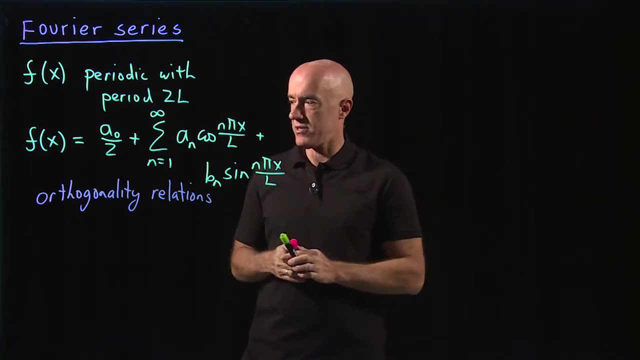 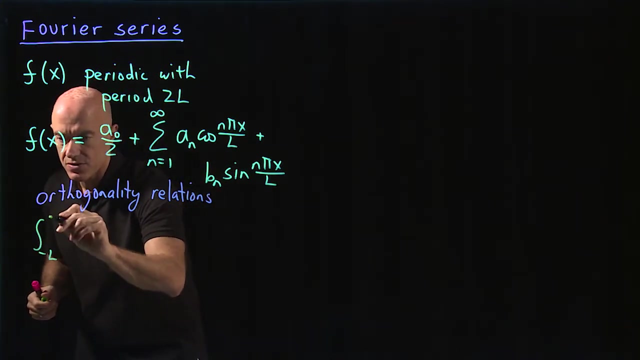 in terms of this function f of x. To determine them, we use some things, some relations that are called orthogonality relations, And those are relations concerning these cosine and sine functions. So let me write down what they are. If you integrate from minus L to L, a cosine function, 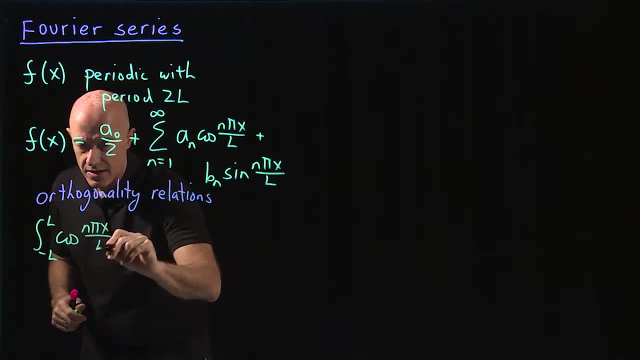 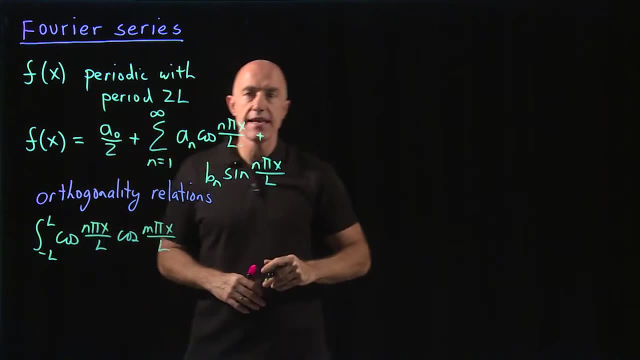 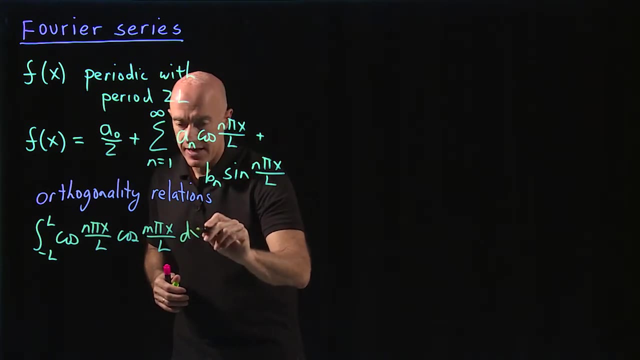 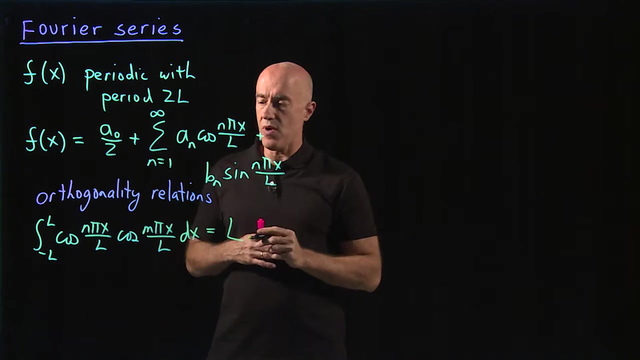 cosine n pi x over L Times, a cosine m pi x over L where n and m are two different positive integers. say: And we integrate this dx, What you get is L, but you only get L when n and m are equal. 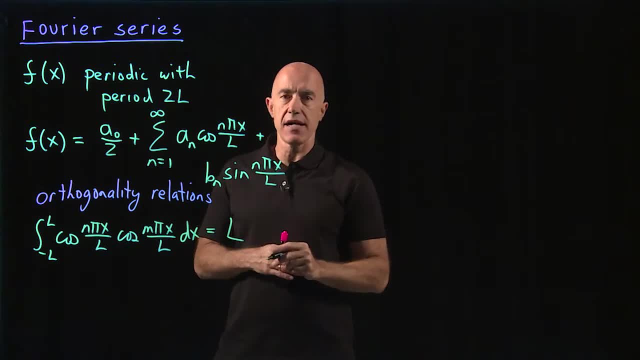 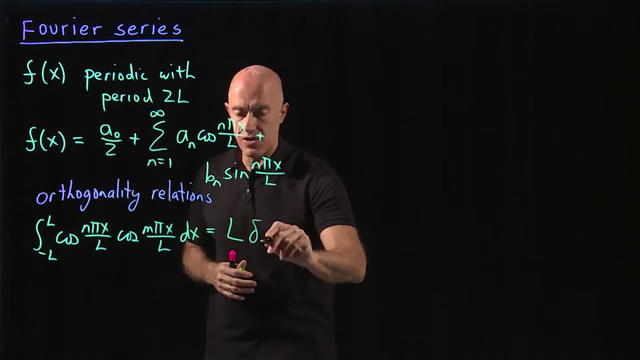 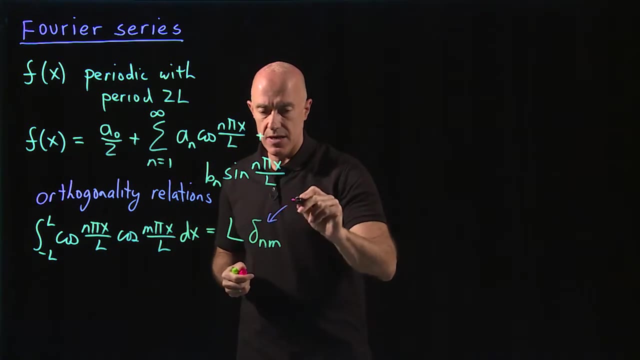 Otherwise you get 0.. That's called the orthogonality relation. Because n and m are not equal, you get 0.. To represent that, we use something called the Kronecker delta. So this piece here, this function here, is called the Kronecker delta. 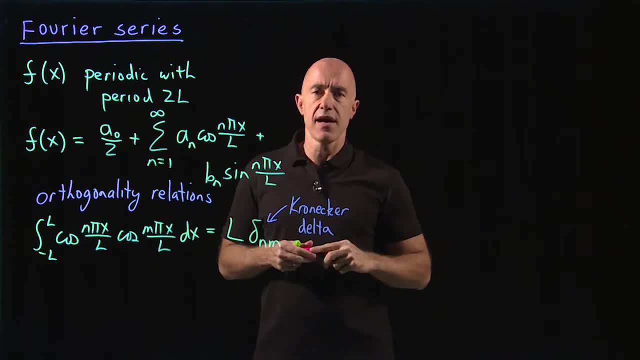 And it satisfies that delta nm is equal to 1 when n equals m and 0 when n is 0. The integral for this n is equal to m. So this is an orthogonality relation for these cosine functions. You can prove this by doing the integral. 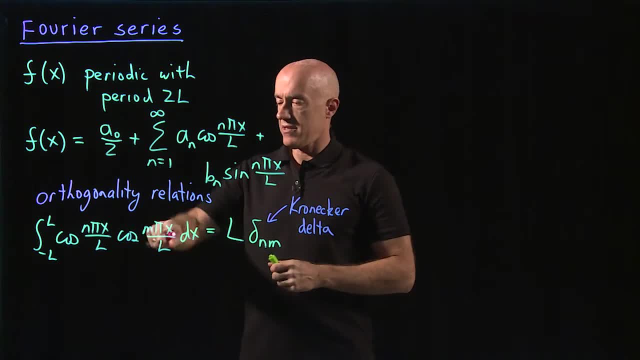 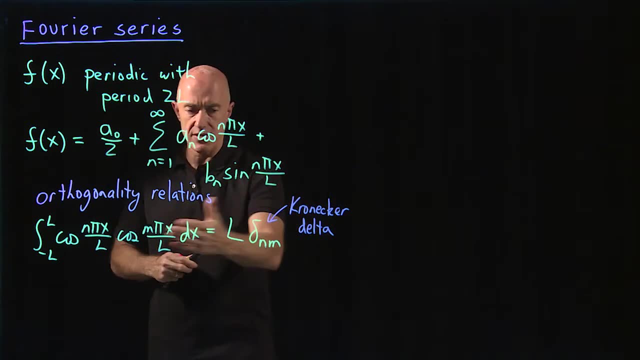 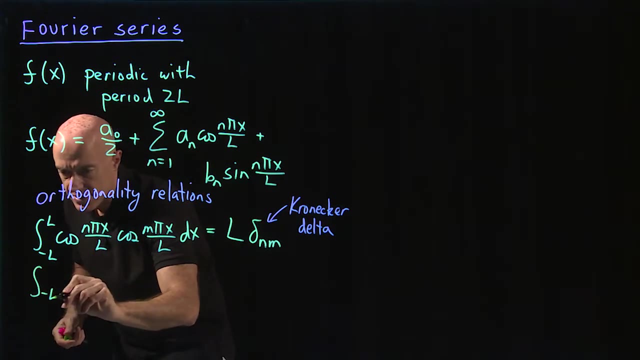 Many of you have done a cosine squared type of integral in calculus. I won't do that here. We'll just assume that one can do this integral. The other orthogonality relations are the integral for minus L to L, sine n, pi x over L. 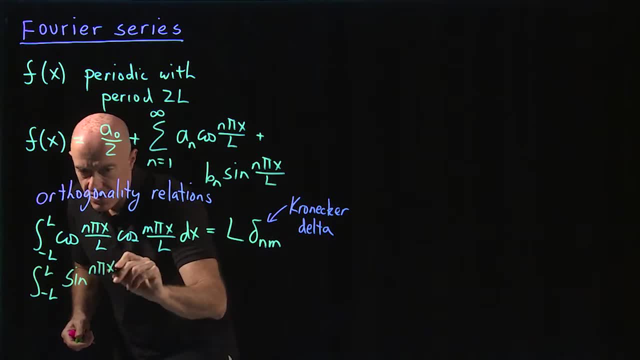 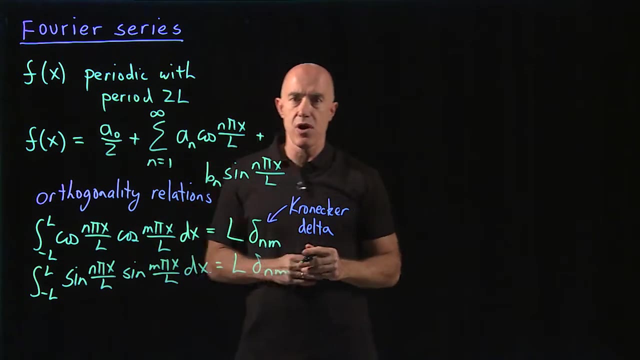 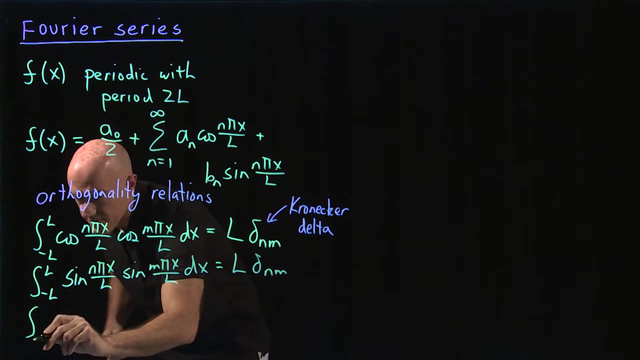 and integral for a cosine function, cosine npi x over L, and integral for a cosine function sine n pi x over l, sine m pi x over l dx, and that again is equal to l times delta n- m when n and m are positive integers. and the last orthogonality relation is the integral from: 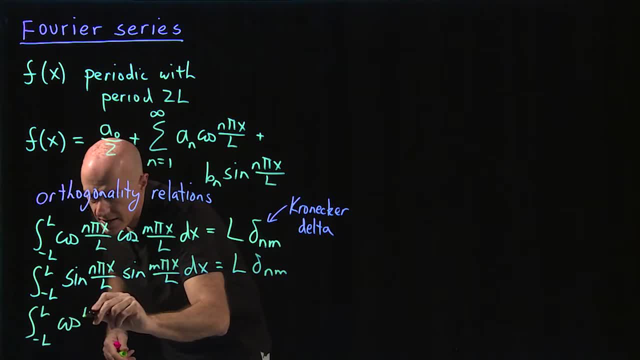 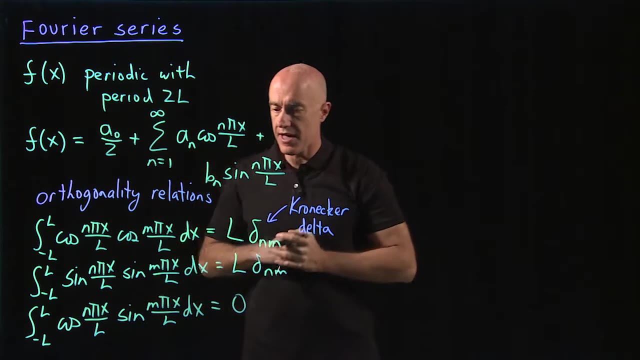 minus l to l of a cosine n pi x over l times a sine m pi x over l dx, and that's always equal to zero. Using these relations we can solve this Fourier series for the a coefficients and the b coefficients. I can give you one example of how that would work. 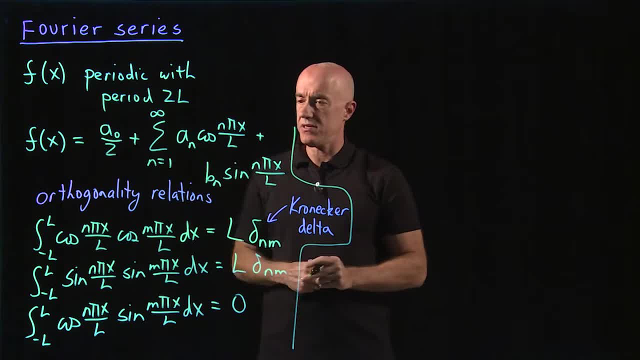 Let's say we wanted to find the b coefficients. To find the b coefficients what we would do is we would multiply, we would integrate the left hand side, So we'd take the integral from minus l to l of f, of x. And we want to find b sub n say: 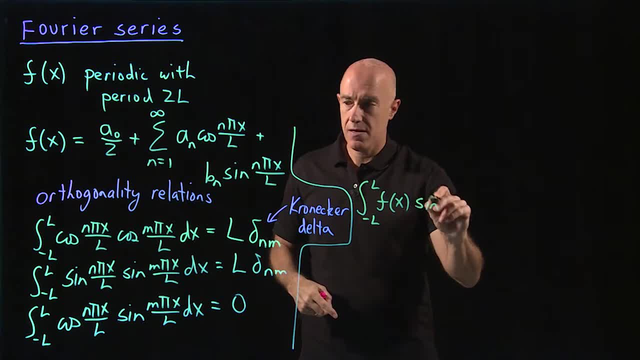 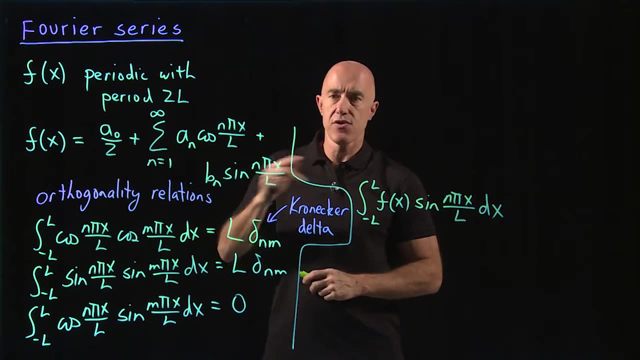 So we would multiply by sine n pi x over l and integrate. And then what would happen? So if we multiply this constant by sine n pi x over l and integrate dx, we would get zero. That term would go to zero If we multiply this constant. 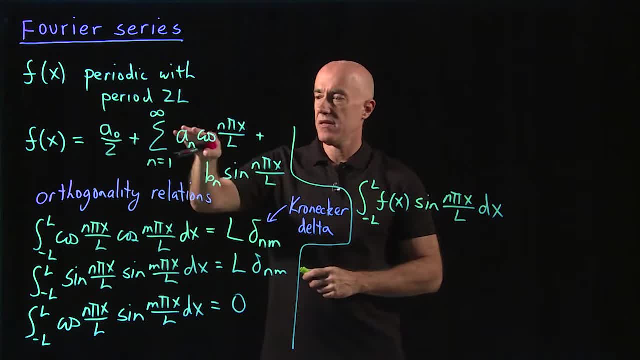 We would get zero If we multiply this cosine by a sine. we would have to change this dummy variable in the summation. instead of saying from n equals one to infinity, we would have to choose m equal one to infinity, And then this would be a sub m cosine: m pi, x over l. 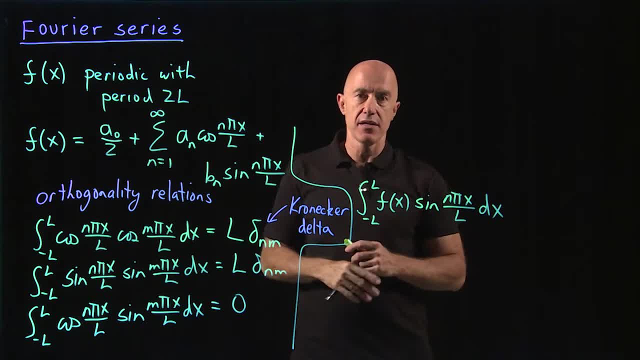 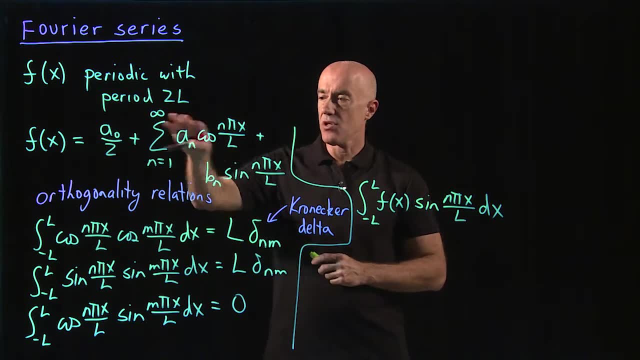 If we multiply by sine n, pi, x over l and integrate dx, then this third orthogonality relation would give us zero. So the only thing we would have left is this last term. So this would be equal to the sum. and then I'm changing the n there to m. 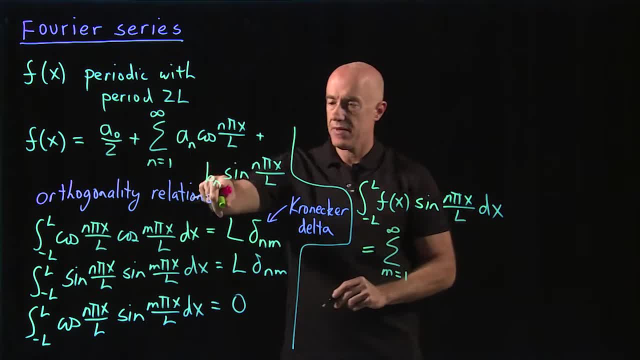 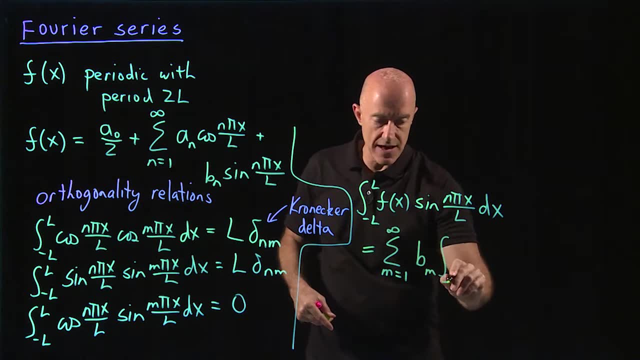 So m equals one to infinity, And then we would have a b sub m, And then we integrate it, So we would have an integral from minus l to l, and then we would have here, we would have our sine, and then we would have x minus m. 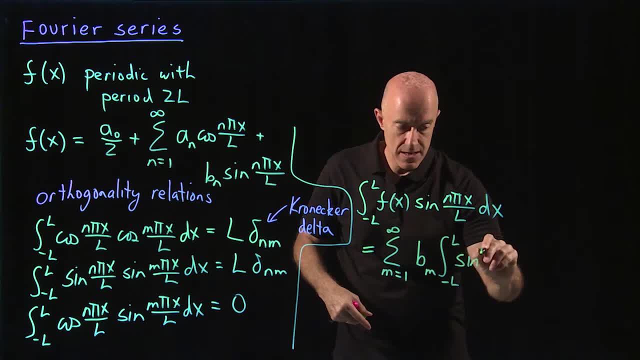 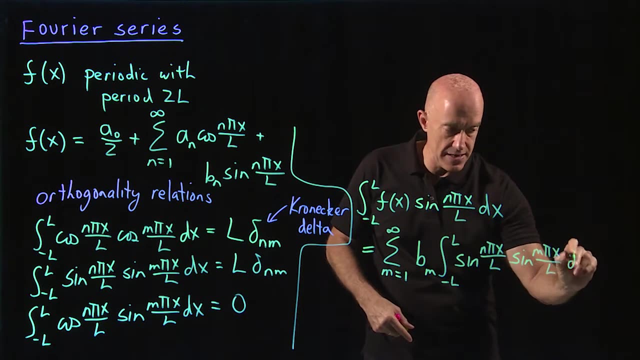 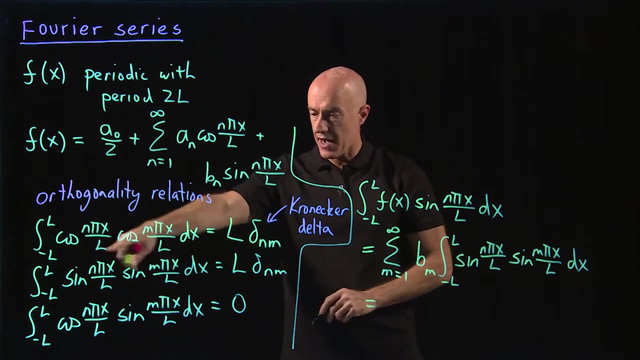 And then we'd integrate, So we'd have our sine, Therefore sine n pi x over L, And from this one, because we changed n to m, we would have a sine m pi x over L and we integrated dx. So now we would make use of our second orthogonality relation. 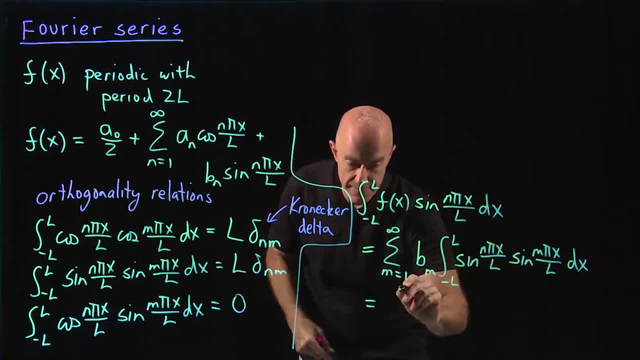 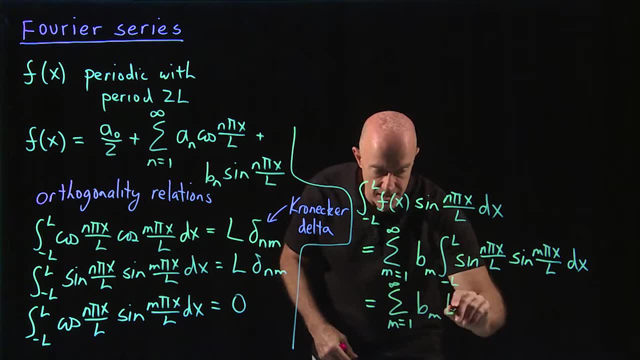 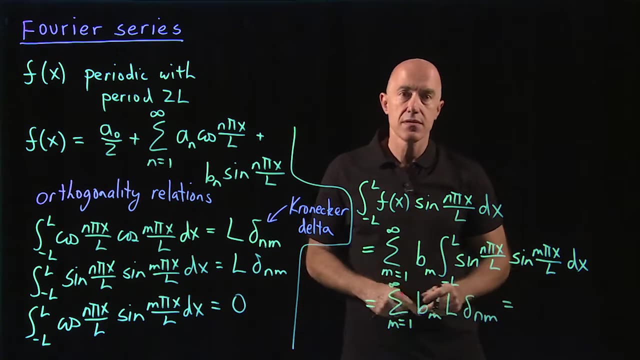 So this integral would be L delta nm. So this would be the sum from m equals 1 to infinity b sub m times L delta nm. And now delta nm is 0 unless m is equal to n. So every term in this sum will be 0, except the term where m is equal to n. and then we 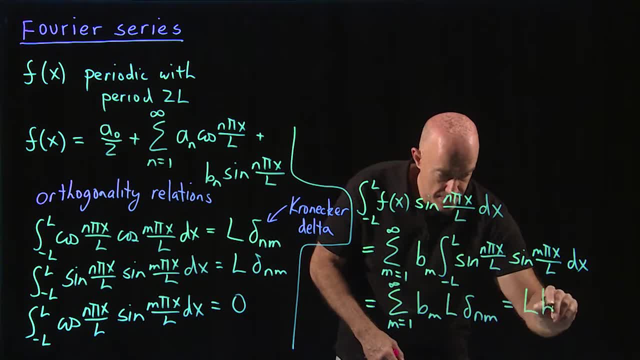 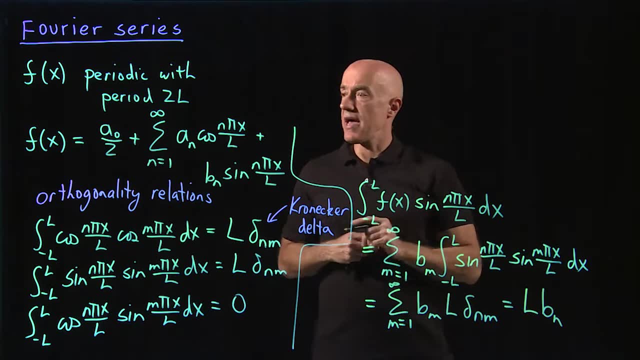 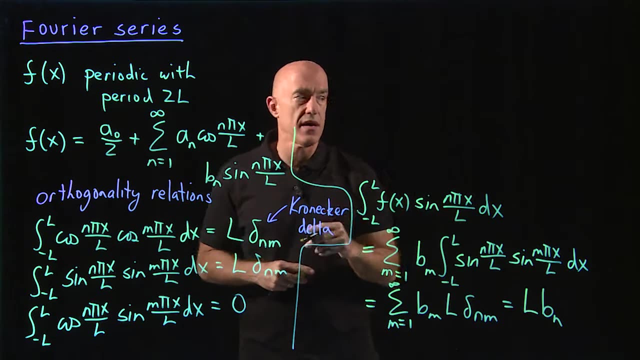 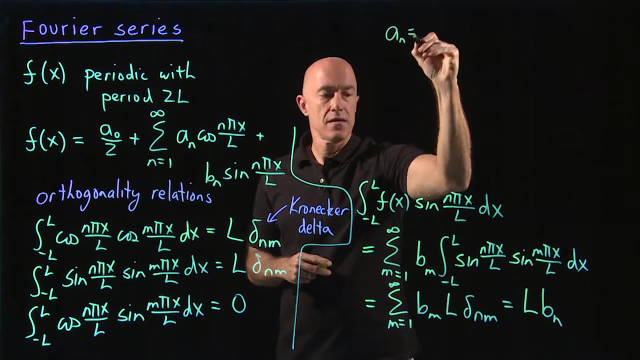 get L times bn, And then we can solve this. We can solve that for bn. OK, so that's how you find the b's, You get the a's the same way. I should just write down what the expressions are. So we have a sub n then is given by the integral, or you have to divide through by L. 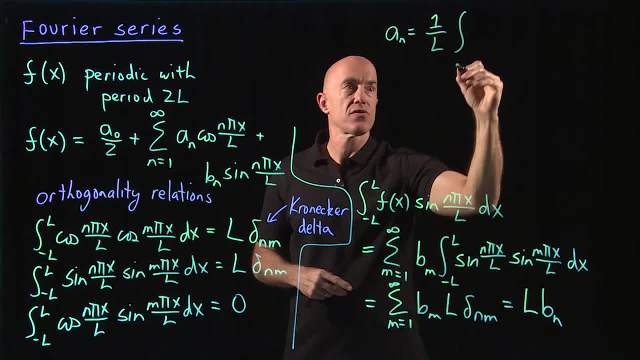 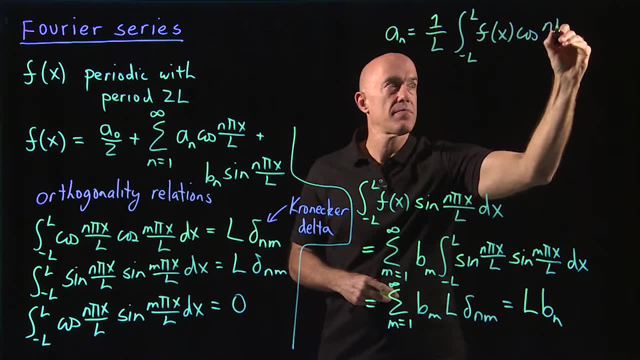 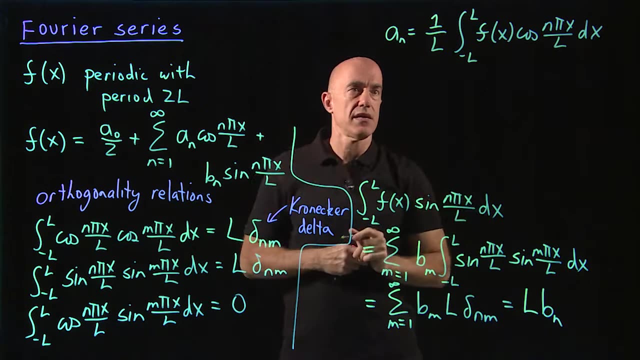 So it's given by 1 over L times the integral from minus L, And it would be f of x times cosine n, pi x over L dx. So a sub n's are given by this integration, and that's also true for a0, the first a coefficient. 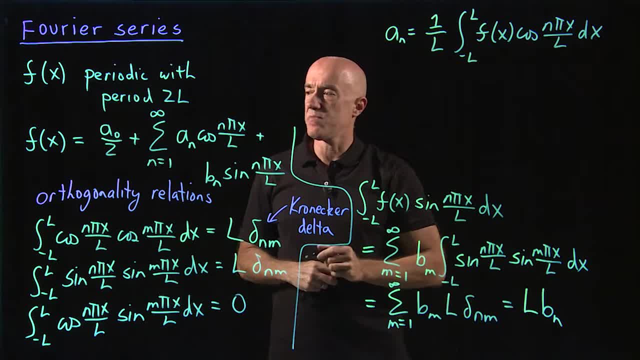 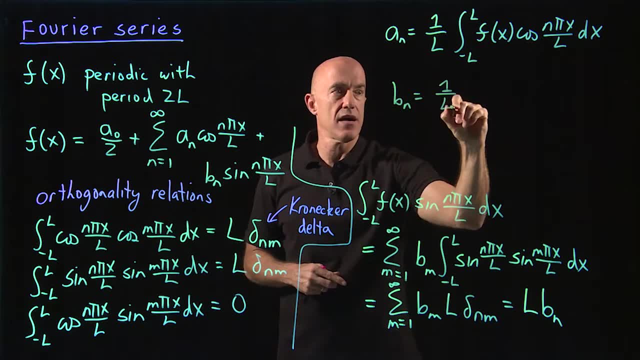 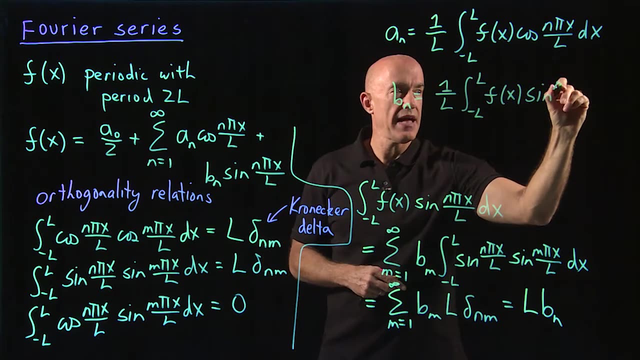 because that's why we stuck the 2 there, so that this formula would also work. The other one then would be: b sub n equals 1 over L dx. So the integral from minus L to L of f, of x sine n pi x over L dx. 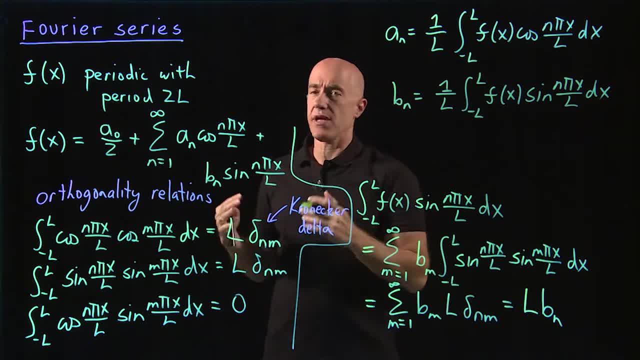 OK, the mathematics of Fourier series is more complicated than this. One has to consider when the Fourier series converges to the function, things like uniform conversions and other mathematical problems. But I think engineers basically are users of Fourier series. They don't need to understand too much theory. 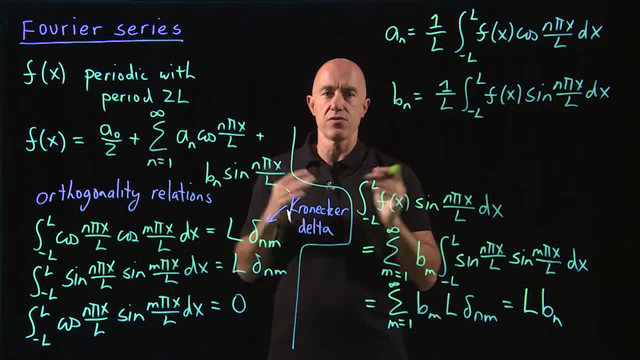 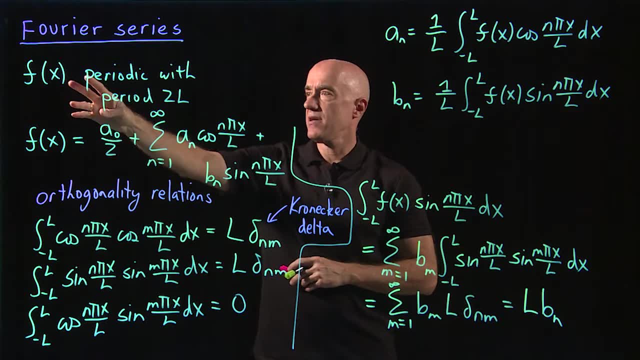 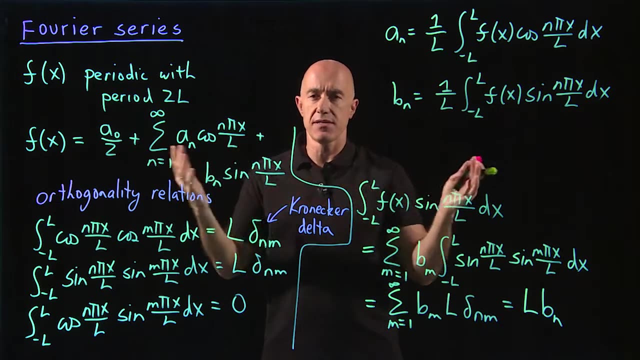 So let me explain to you, let me review for you then, what you do need to understand. So we're talking about representing a function f of x, that's a periodic function with a period of 2 times capital. L- L is typically some related to some length of the system. 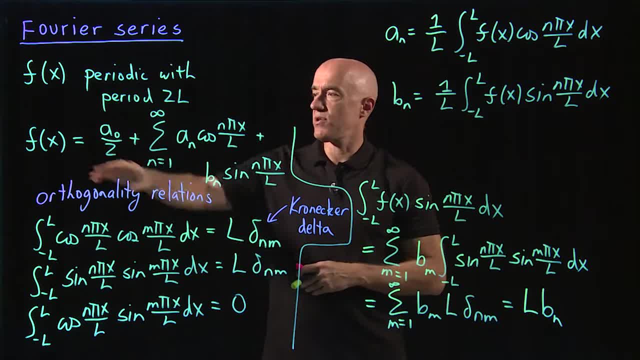 We write the Fourier series as: f of x equals a0 over 2, a constant term plus the sum from n equals 1 to infinity, of a sub n times cosine n pi x over L, plus b sub n times sine n pi x over L. The use of the cosine and the sines ensure that this function is periodic with.